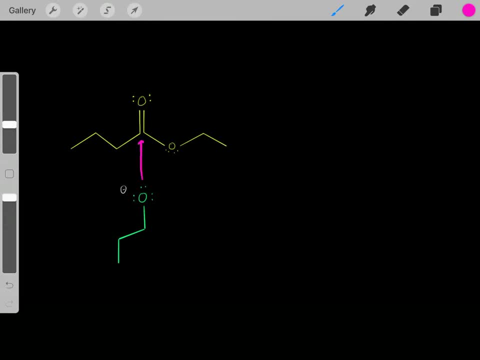 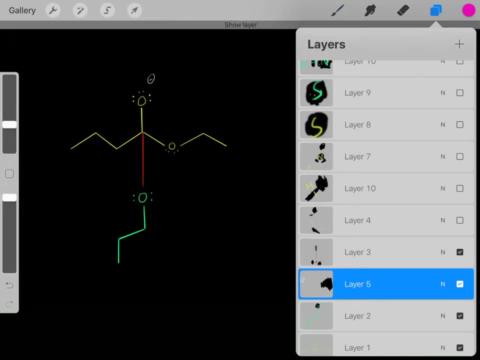 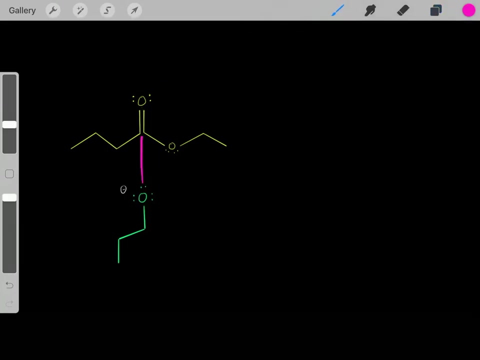 attack this carbon. When we attack, we form a bond, and once we form a bond, we push these pi electrons up onto this oxygen. When we do that, we'd essentially form this tetrahedral intermediate where, again, we attack. remember what we did: We attacked, we formed a bond. 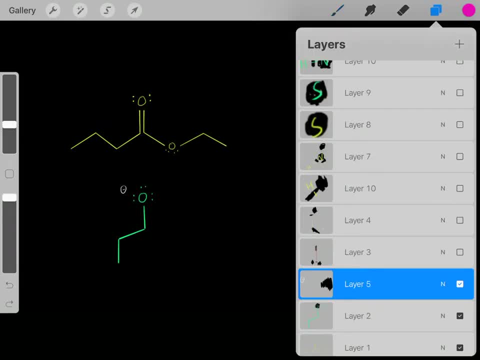 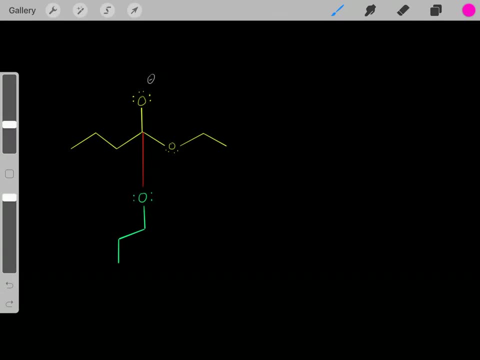 and when we formed that bond, we pushed these pi electrons up onto this oxygen, forming this tetrahedral intermediate with this oxygen anion. So now, once we form this tetrahedral intermediate, we know this is unstable with this formal charge of negative, one that's. 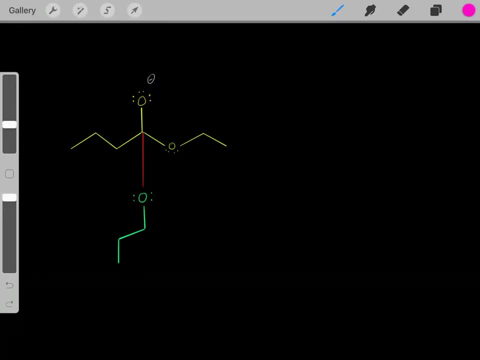 not stable. So now what happens? are these electrons essentially scoop down? They scoop down forming a double bond and once they do that, now this bond breaks where these electrons fall, in this oxygen. So again these electrons scoop down, forming that double bond. When we do that, 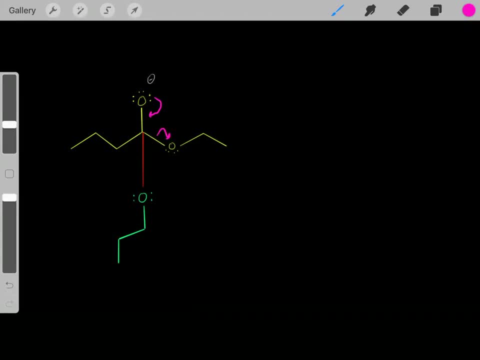 this bond breaks where these electrons fall in this oxygen. So again we form a double bond and we break this bond. So when we do that, we'd essentially form this product. So now we've done it, We've formed a bond. 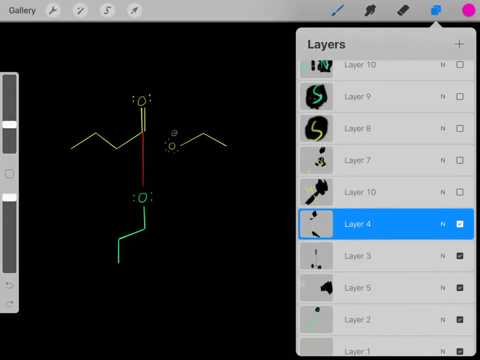 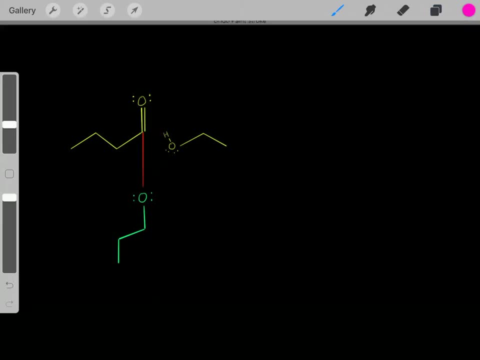 and we broke this bond, Then this isn't stable And, depending on the mechanism, it would get pertinent at some point. But again, soon as we've done it, we formed a bond and we broke a bond And this is a very common mechanism. you'll see over and over again in biochemistry. 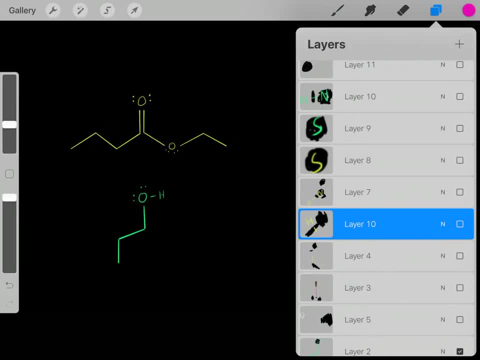 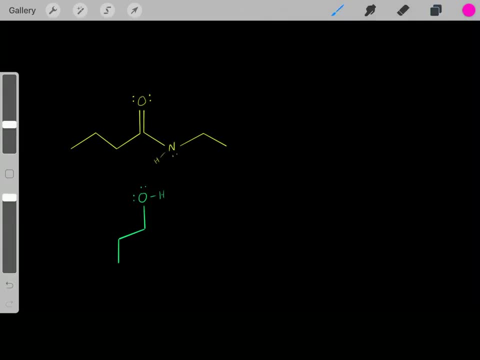 And in fact you'll see slight variations. For example, instead of this being an oxygen with this ester, maybe we'll have some kind of amide or amido. So again, it's the same idea, where again we can take this oxygen and essentially form a bond. And once we form a bond, we break this bond. 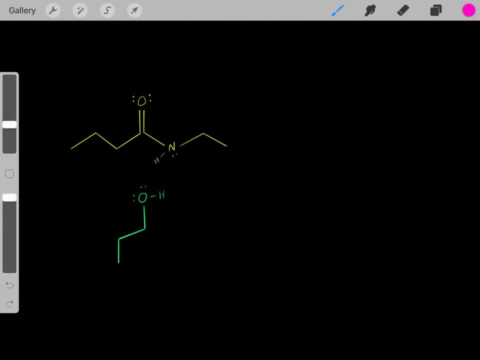 with these electrons falling on this nitrogen. But again, it's the exact same mechanism, the exact same thing. The only difference is: instead of an oxygen, this is a nitrogen. And again, when it gets protonated or not, but again same idea. First step: we create a stronger nucleophile. 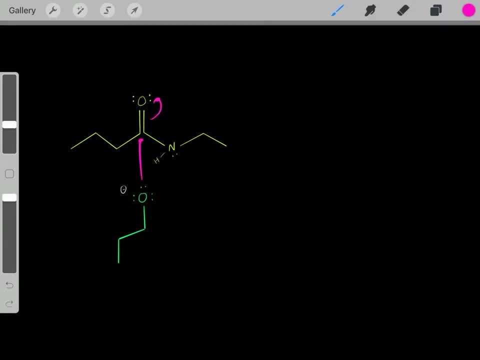 Now we nucleophilically attack, forming a bond. We push these pi electrons up on this oxygen. When we do that, we form this tetrahydroner mediate. Now the electrons scoop back down, forming a double bond And when that happens we break the bond with an ester. 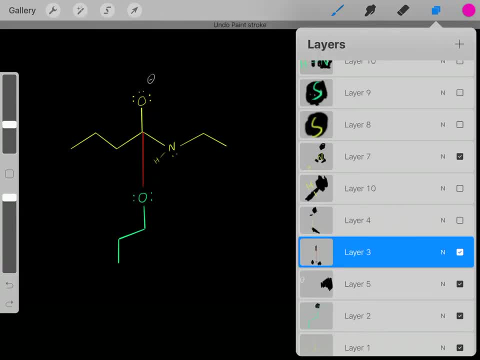 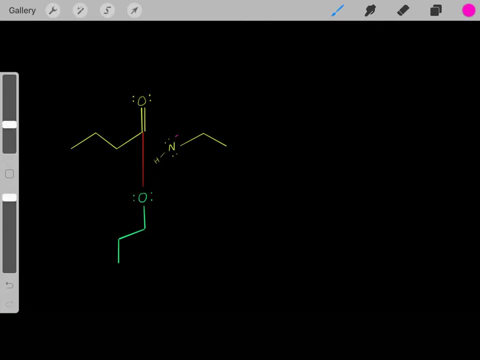 happens Now this bond breaks, these electrons fall in this nitrogen. When we do that, we again have our product where again we formed a bond and we broke a bond, And again this would be negatively charged. but the point is that then it would get protonated, But again we formed a bond. 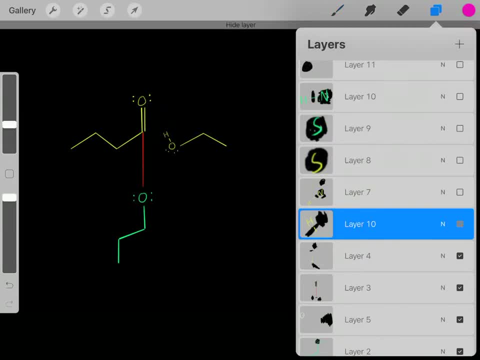 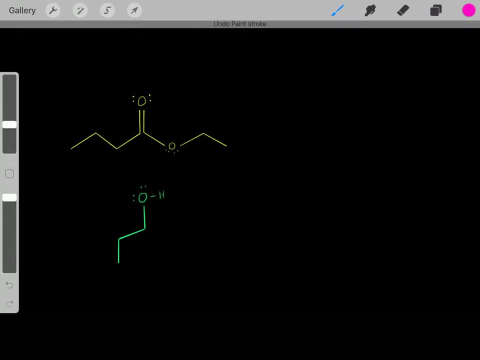 and we broke a bond and it's that exact same mechanism And you'll see the same general mechanism over and over again in biochemistry, And again we know this could be an oxygen, It could be a nitrogen, It could also be a sulfur, It could also be a sulfur, but again it's the. 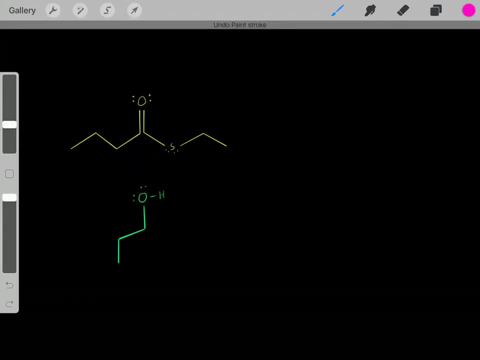 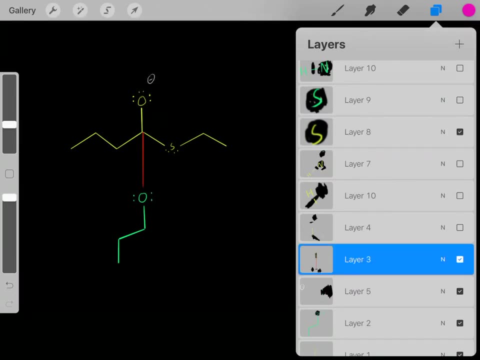 exact same mechanism: We form a bond, we break a bond. And again we know how we do this. now Create a strong nucleophile. We nucleophilically attack, forming that tetrahedral intermediate, Then electrons scoop back down, forming that double bond, breaking this bond, These electrons. 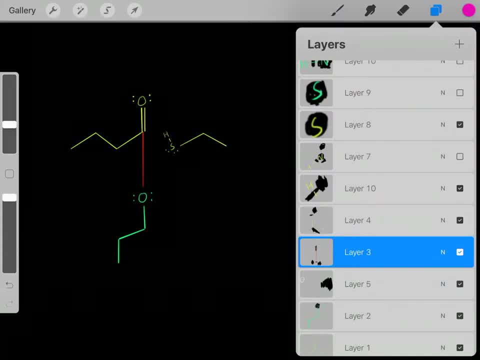 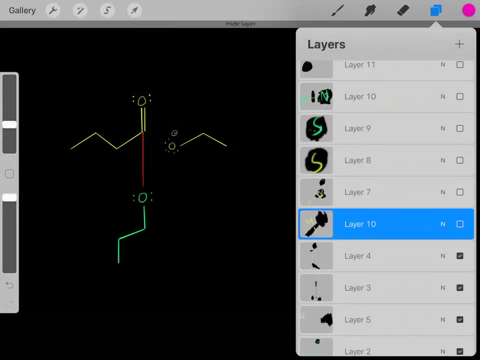 fall in the sulfur. When we do that now, we form this and then the sulfur would get protonated And again we formed a bond and we broke a bond. So you'll see, now that you understand and seen this mechanism, you'll see this mechanism over and over again in biochemistry. 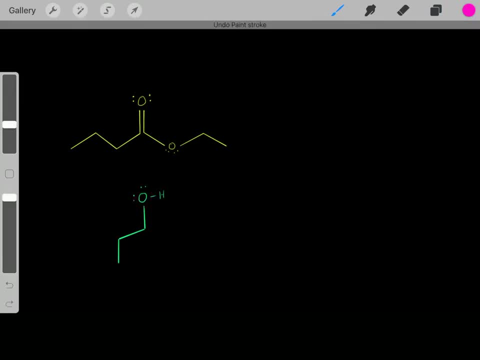 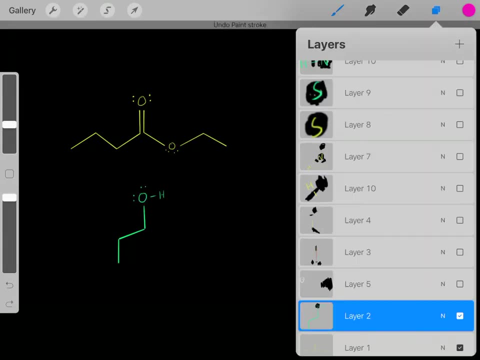 But we can also change it based on what this nucleophile was In all these examples, whether this was oxygen, nitrogen or sulfur, we could have done all the same mechanisms, but instead of an oxygen. instead of an oxygen, maybe we had a sulfur nucleophile, But again. 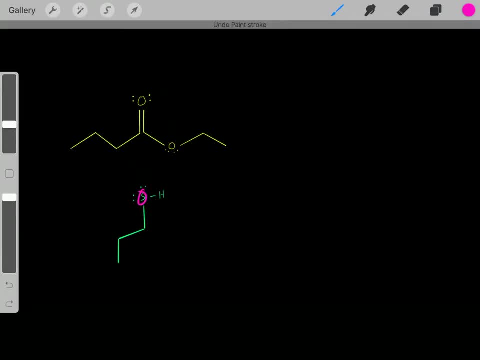 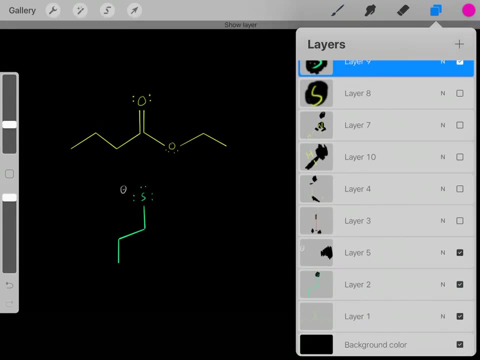 it's the exact same thing. Imagine those exact same steps. but instead of an oxygen, now we have a sulfur. So again, first step: create a stronger nucleophile. Now we have a stronger sulfur nucleophile with that localized negative charge. Then it's the exact same thing Nucleophilically. 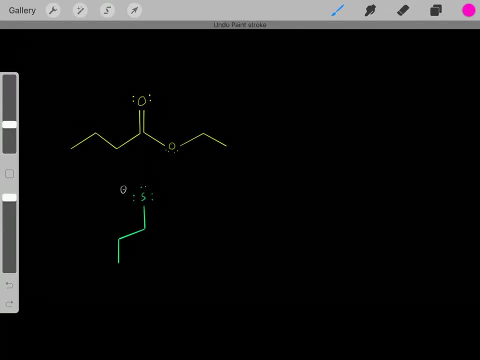 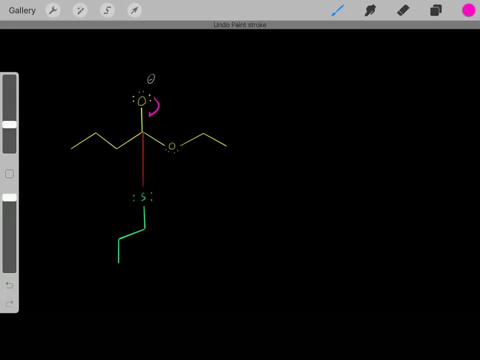 attack, forming a bond, pushing these pi electrons up on this oxygen. When we do that, we form this tetrahedron intermediate. Then the same thing: electrons scoop back down, forming a double bond. Now this bond breaks, these electrons fall on this oxygen. And when we do that, now we form this. 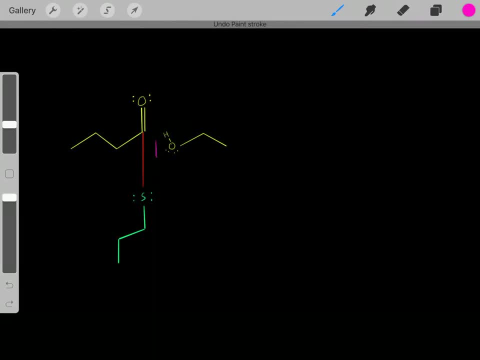 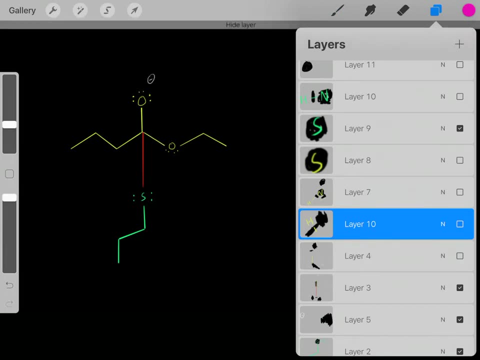 and then again the oxygen will get protonated. But again, we formed a bond and we broke a bond. but it was that exact same organic chemistry mechanism. So it's really redundant. You'll actually see this over and over again in biochemistry. It's the same tricks, But now. 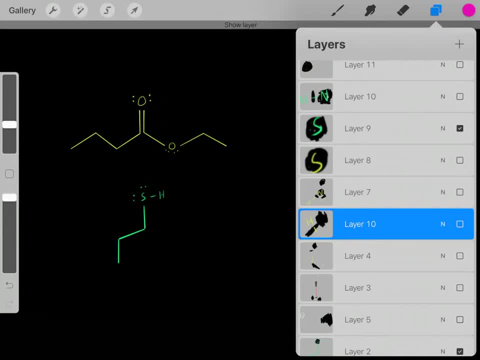 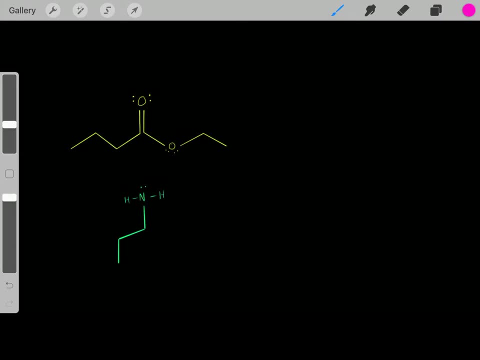 we saw, it can be an oxygen Nucleophile, it could be a sulfur nucleophile, but it could also be a nitrogen nucleophile. And if it's a nitrogen nucleophile, how does this mechanism work? Again, it's the exact same thing. First step, create a stronger nucleophile, Then we nucleophilically. 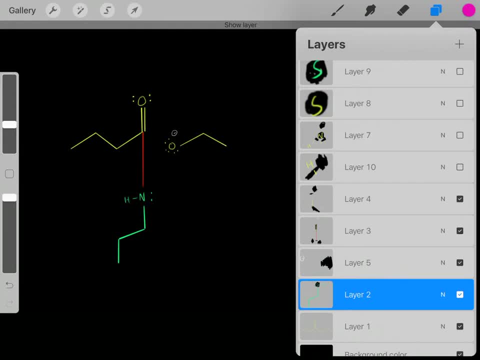 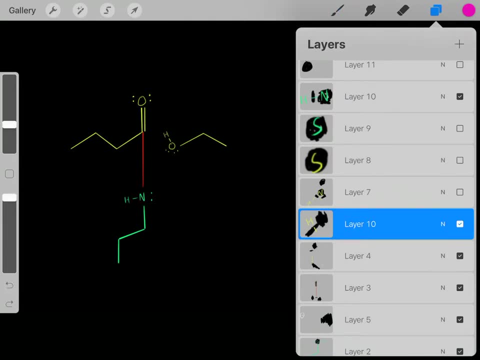 attack forming a tetrahedron intermediate, Then the intermediate collapses, Then this guy gets protonated. But again, we formed that bond and we broke that bond. So the point is, you'll see the same general mechanism over and over again. 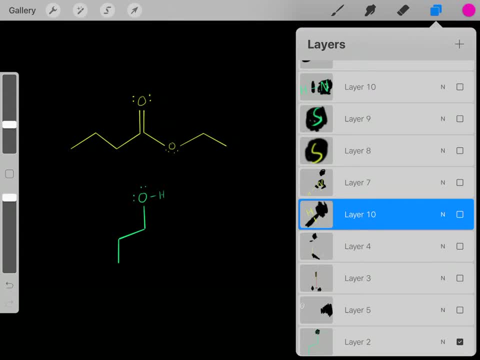 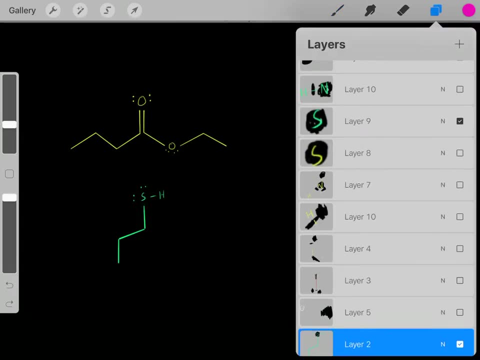 but it's a variation. For example, we know we can have variations in the nucleophiles. For example, we saw we had an oxygen nucleophile. We can also have a sulfur nucleophile, or we could also have a nitrogen nucleophile. So we had variations in this particular nucleophile and we also had 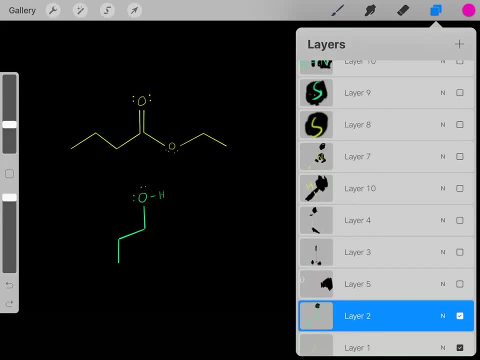 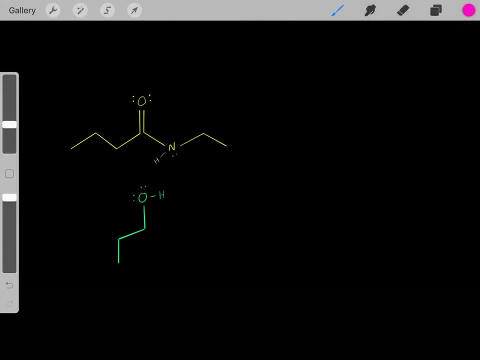 variations on this particular bond. Here we have an ester, but we can also have a thioester, And we can also have this amidotype bond. But again and again we can have combinations. For example, maybe we can have this amidotype. 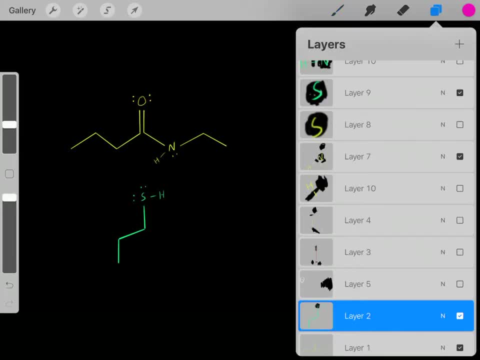 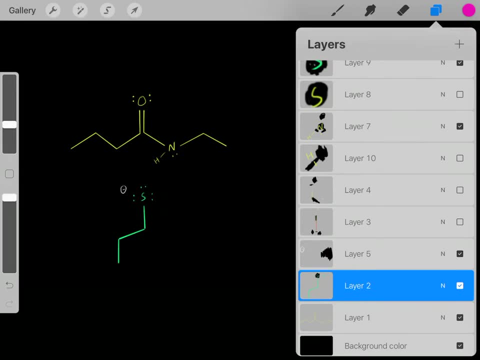 And maybe we can have a sulfur nucleophile. But again it goes to that exact same mechanism. We form a bond and we break a bond And again, first step: create a stronger nucleophile, Then we attack, Then the tetrahedron intermediate collapses, where again then this guy would get? 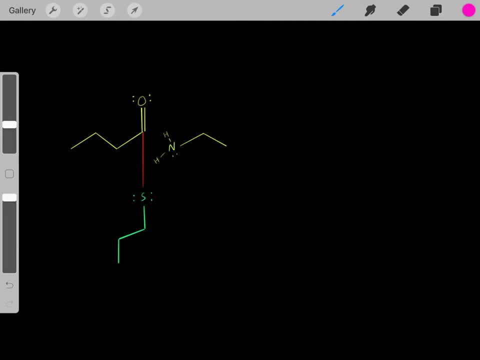 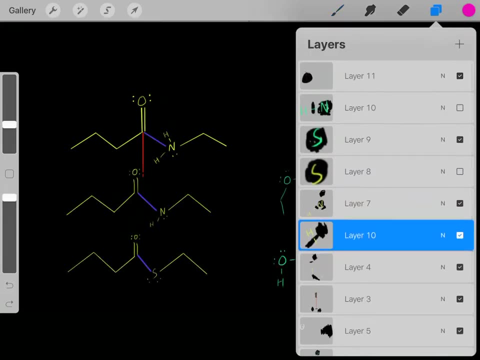 protonated, But again it's that same idea, And so it just varies based on the atoms, whether it's an oxygen, nitrogen or sulfur, But again it's that exact same mechanism, And you'll see these mechanisms over and over again. 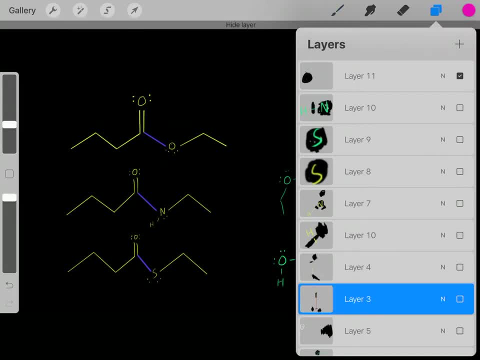 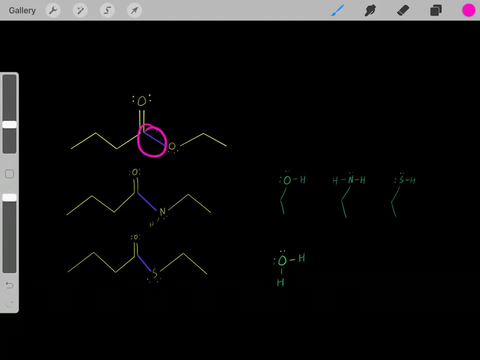 And what's important, essentially, is to realize that again there are these, these. these are three major types of bonds. you'll see in biochemistry, You'll see. you'll see these ester bonds, You'll see these, these amidobonds, And you'll see these thioester bonds, over and over again And you'll. 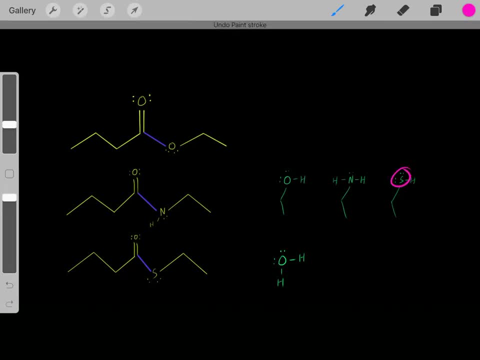 see these different nucleophiles, whether it's an oxygen nucleophile or nitrogen or sulfur nucleophile. And again, instead of this kind of organic alcohol, we could have also, you know, simply had a water molecule. But again we have these different nucleophiles and these different. 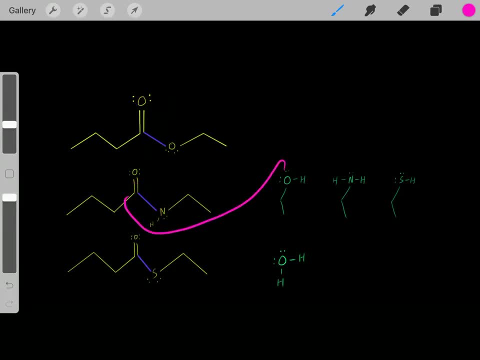 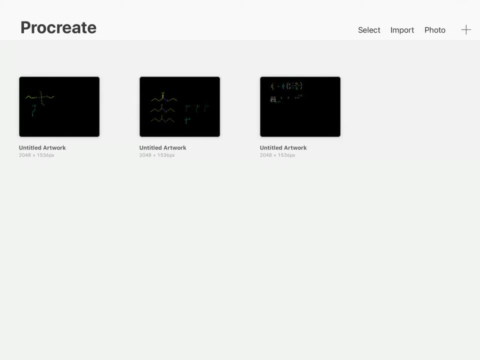 bonds and we can have lots of different combinations. This can break this bond, Or maybe this guy could break this bond, Or this guy could break this bond, etc. We can have lots of different combinations. So that's one common type of mechanism you'll see in biochemistry, But 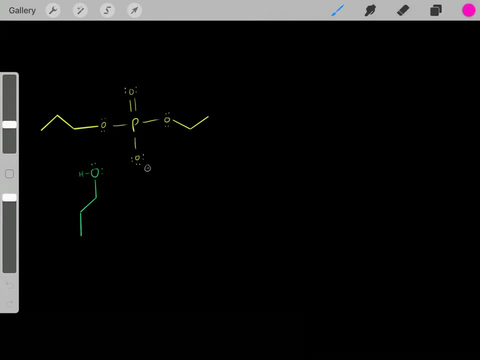 another very common mechanism is again breaking these, these phosphoester bonds, Where again it's the same idea: We form a bond and then we break a bond. So again same idea And something, and the first step is again, this is our nucleophile. So first, 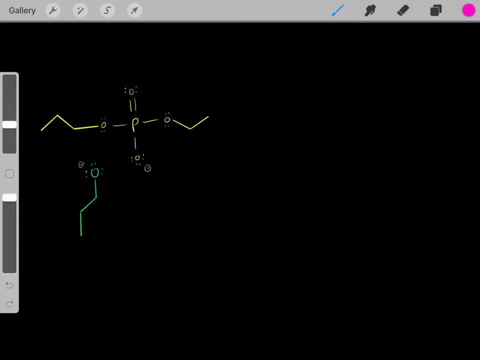 step is we create a stronger nucleophile. So with this localized negative charge, So now we have a nucleophile And also we know this phosphate is electrophilic. Well, how do we know this phosphate is electrophilic? Well, look at all these very electronegative oxygen atoms it's bonded to. 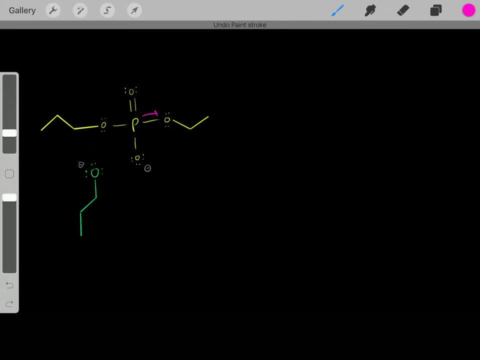 All these oxygens are pulling electron density because they're more electronegative, So therefore we have a strong electron deficiency on this phosphorus. So now we have an electrophilic phosphate phosphorus. So now we have an electrophilic phosphorus. So now we have an. 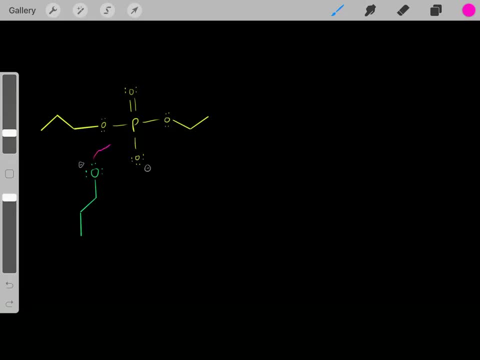 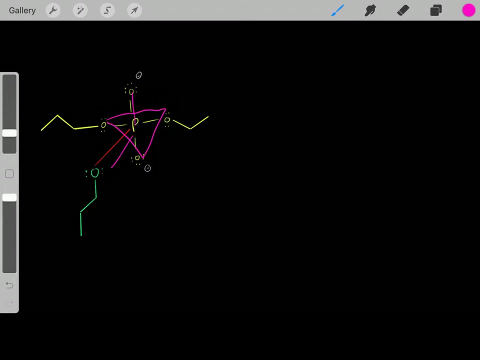 electrophile and a nucleophile so they can react. We nucleophilically attack. When we attack, we form a bond, And when we form this bond, we push these pi electrons up on this oxygen. When we do that, we form this intermediate, which is referred to as a trigonal bipyramidal. 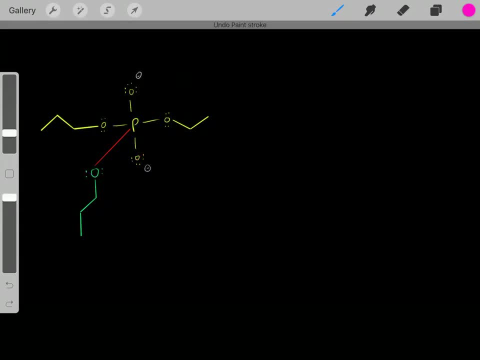 intermediate. And again, the geometry isn't very precise here, but the more precisely the geometry would look like this: Where again we have this triangle, this trigonal, and then we have this bipyramidal. So this is more accurate, the geometry, what the geometry looks like, Where. 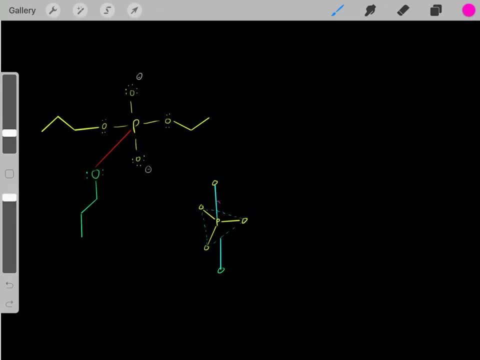 again we have these 60 degree angles and then this is perpendicular, But again we form. the point is: the point is we form this trigonal bipyramidal intermediate. Then once we form this intermediate, then these electrons scooch back down. When they fall back down, they form a double. 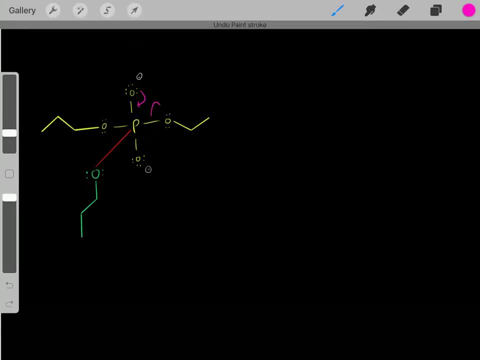 bond And when that double bond is formed now we break this bond with these electrons falling on this oxygen. When we do that, we'd essentially form this Product Where again we formed a bond and we broke a bond. So I know this reaction is a little. 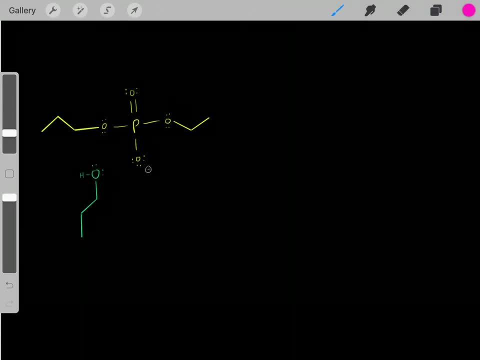 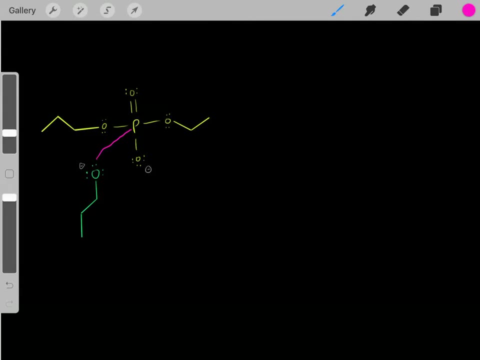 complex. This mechanism is a little intimidating, but let's do it again. Remember: first step: we create a stronger nucleophile. Now the nucleophile nucleophilically attacks, Forming a bond. we form a bond And once we form that bond, we push these pi electrons up on this oxygen. 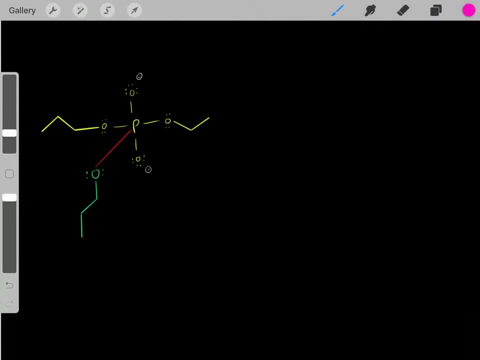 So when we do that, we form, remember this trigonal bipyramidal intermediate. We formed a bond and then we push those pi electrons up on this oxygen, Forming this trigonal bipyramidal intermediate. Now, once we form this intermediate, now we know, 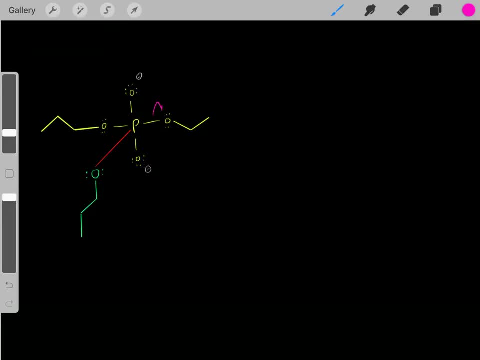 the electrons scooch back down, forming a double bond, breaking this bond, with these electrons falling on this oxygen. When we do that now, we'd essentially form this where we broke this bond. So we formed a bond and we broke a bond, And this is another very common mechanism you'll see in 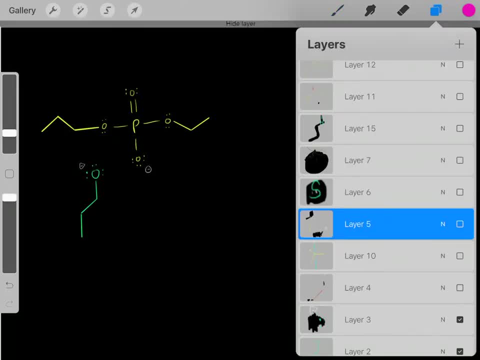 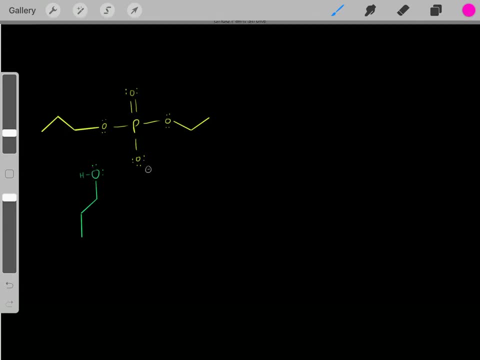 biochemistry. But again, just like we talked about earlier, we can have lots of different nucleophiles. We can have an oxygen nucleophile, We can also have a nitrogen nucleophile, Or instead of a nitrogen nucleophile we could have a sulfur nucleophile. 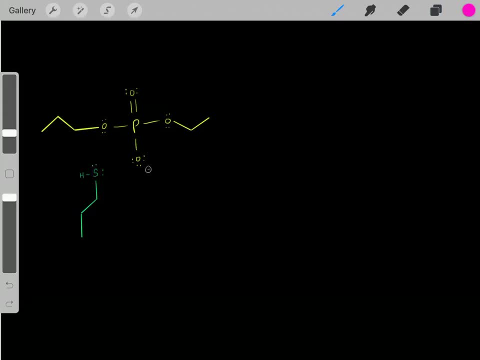 Again, we could. whether it's sulfur or oxygen or nitrogen, it's the exact same mechanism. First step: we create a strong nucleophile. Now we nucleophilically attack, forming a bond, pushing these pi electrons up on this oxygen. So when we do that, remember we form this. 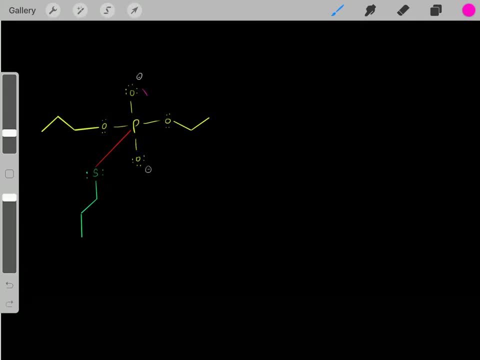 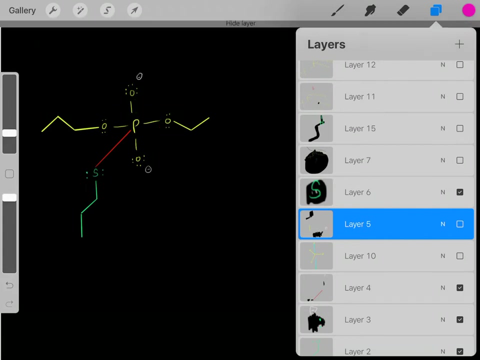 trigonal bipyramidal intermediate. Then the electrons fall back down, forming that double bond, breaking this bond. These electrons fall on this guy. So when we do that, we form our product, We form a bond bond and we broke a bond. But again, it doesn't matter what kind of original nucleophile you had. 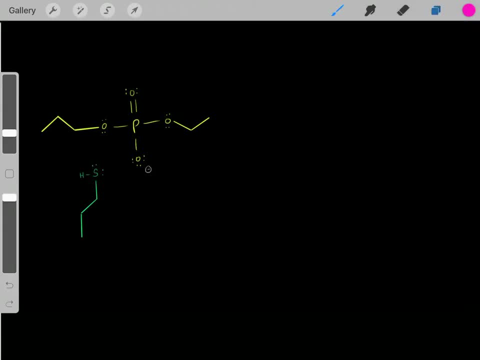 whether it was a sulfur nucleophile or an oxygen nucleophile or a nitrogen nucleophile, etc. It's that exact same mechanism And you'll see this mechanism of a nucleophile forming a bond with one of these phosphoesters and then breaking a bond. You'll see that over and over again in 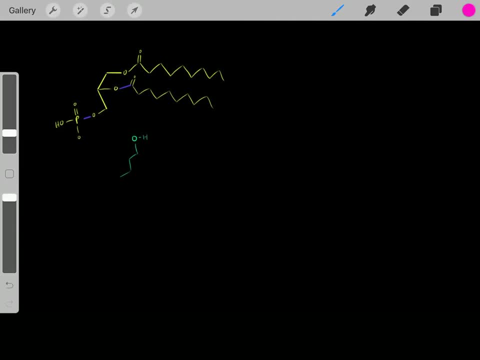 biochemistry. Now that you know this, you'll recognize it. So, for example, a very common macromolecule in biochemistry are these phospholipids, where we have this glycerol backbone and these fatty acids and this phosphate. But again now with our mechanisms that we know. 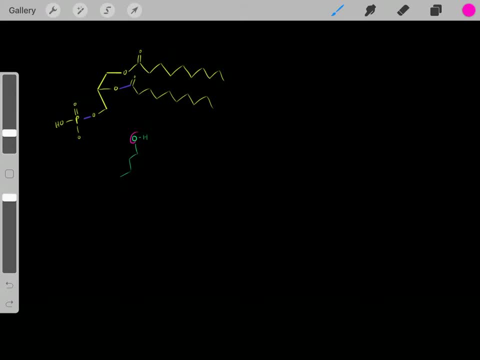 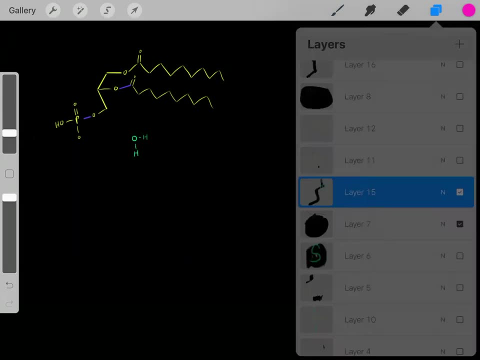 we know how we break these bonds. We know how we break these bonds, For example, whether we have an oxygen nucleophile or a nitrogen nucleophile or sulfur nucleophile. And again, for simplicity, let's just create a very simple oxygen nucleophile as in water. And again we 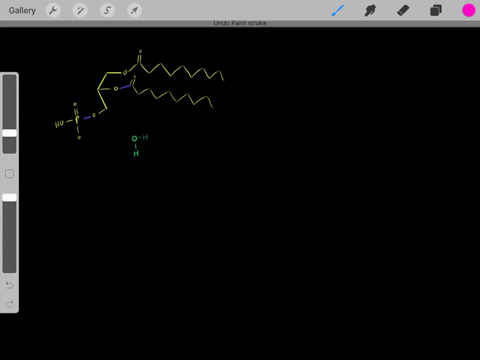 have a lot of water in the cell. so commonly water is the nucleophile. But we know using this water we can form a bond and we can break a bond. And we know we nucleophilically attack, pushing these pi electrons up on this oxygen, forming that tetrahedral intermediate. 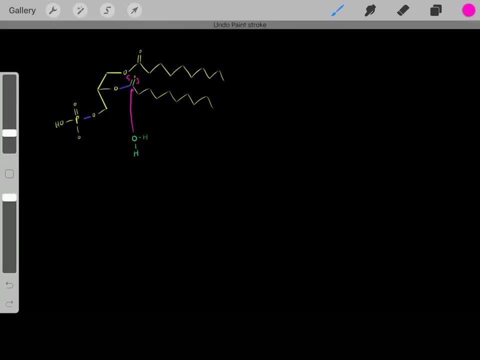 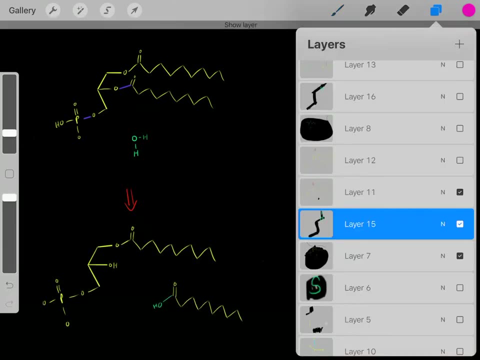 then the electrons scooch back down, reforming that double bond, breaking this bond, with these electrons falling on this oxygen. But again we can essentially form a bond and break a bond, And that's how we hydrolyze those ester bonds. And now we formed our product, where, again 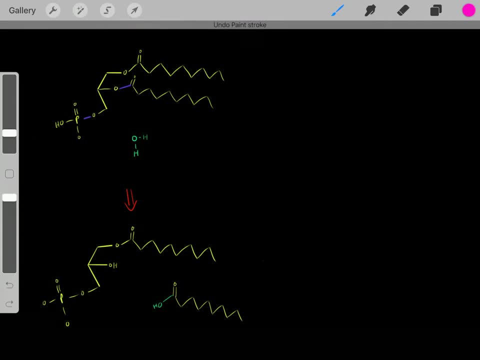 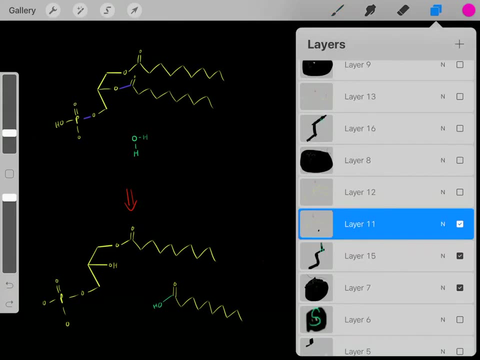 we formed a bond and we broke a bond. So this bond that was formed is represented by this bond. and then we broke this bond. So that's how we hydrolyze these ester bonds in these fats. But not just that. we know we can also hydrolyze this bond where again, 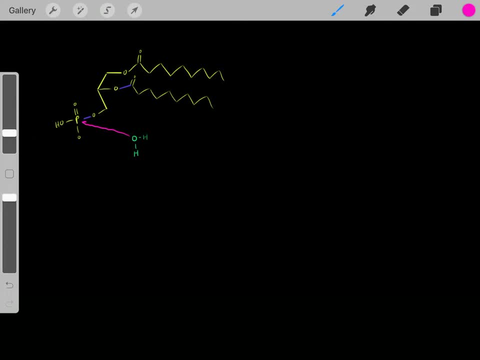 we know this mechanism: we nucleophilically attack, forming a bond. When we do that, we push these pi electrons up on this oxygen, forming that trigonal bipyramidal intermediate. then the electrons scooch back down, reforming that double bond, breaking this bond with these. 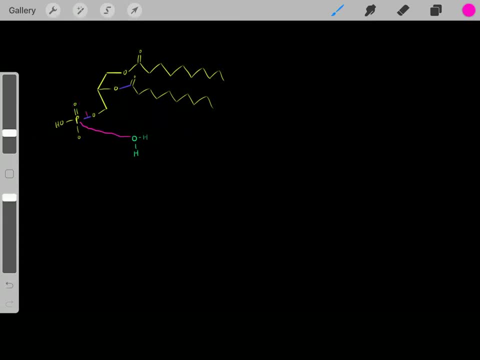 electrons falling on this oxygen. Again we're forming a bond and we're breaking a bond, And when we do that, we'd essentially form this product where again we broke this bond. that's how we hydrolyze these phosphoester bonds, And again it's that same mechanism that we learned. 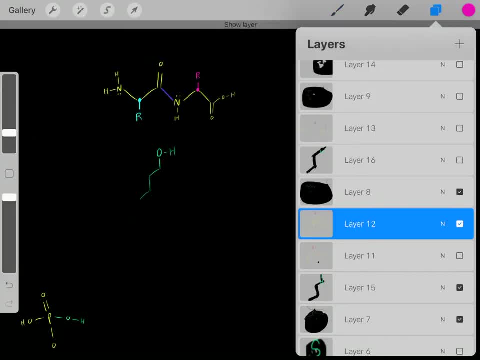 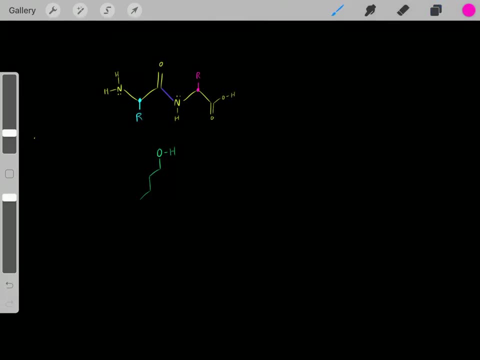 about earlier And you'll see these kinds of mechanisms over and over again. So now let's do another example. Let's do another example. Let's say we have this dipeptide, where we have these two amino acids linked together with one of these peptide bonds. Again, remember, it's one of. 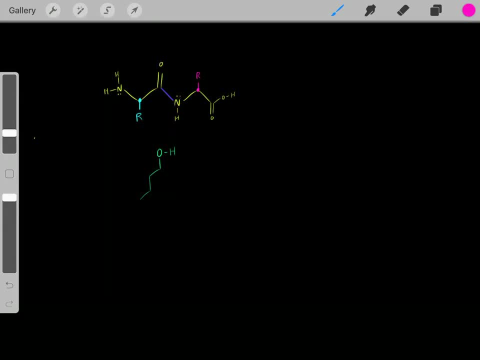 those bonds we saw where, again, whether this is oxygen, nitrogen or sulfur, we know how we break this bond as long as we have a nucleophilic bond. And again we're forming a bond where, again, for simplicity, let's just use a simple water nucleophile. But we know this mechanism, We 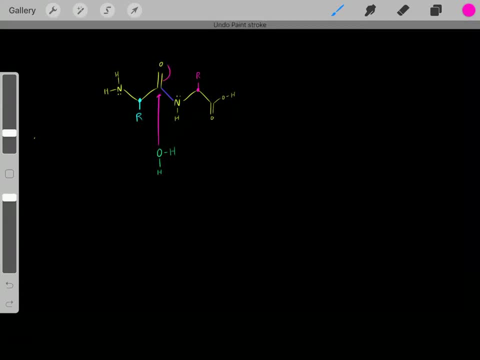 nucleophilically attack, forming that bond. then we push these electrons up on that oxygen, forming that tetrahedral intermediate. then the electrons scooch back down, reforming that double bond. Now we break this bond, these electrons fall on that nitrogen. But again it's that same idea. We form 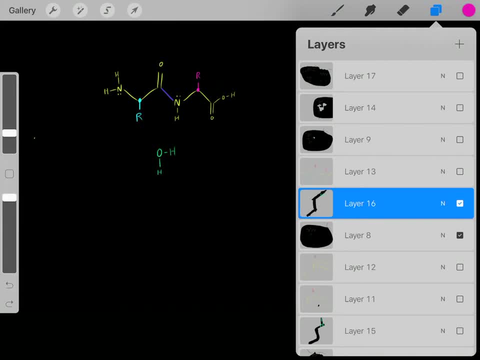 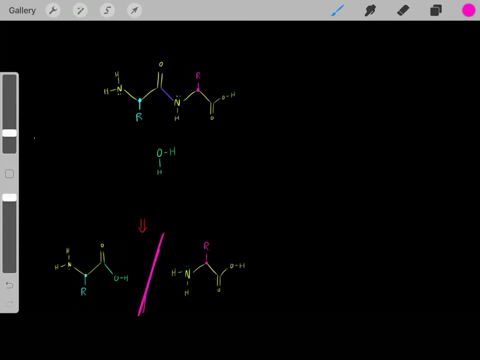 a bond and we break a bond. these electrons fall on the nitrogen, And now we know how we hydrolyze these peptide bonds. That's how we use water molecules to break these peptide bonds, And now we broke the peptide bond. We're going to do another example. We're going to do another example. We're. 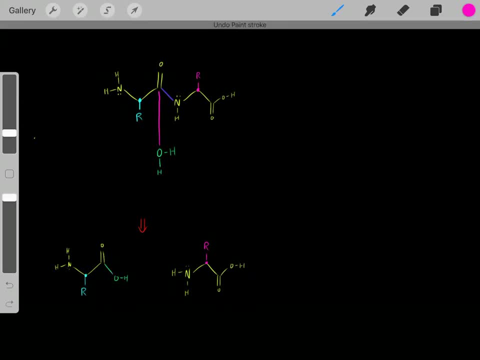 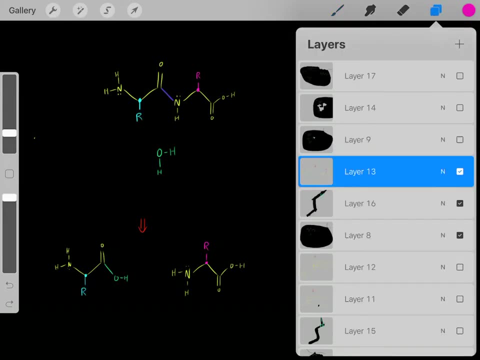 again, we formed a bond and that's represented by this bond, And then we broke this bond, So now we don't have this bond anymore. So that's how we break these peptide bonds, But again it's that same mechanism that we learned about earlier. You'll see these same mechanisms over and over.